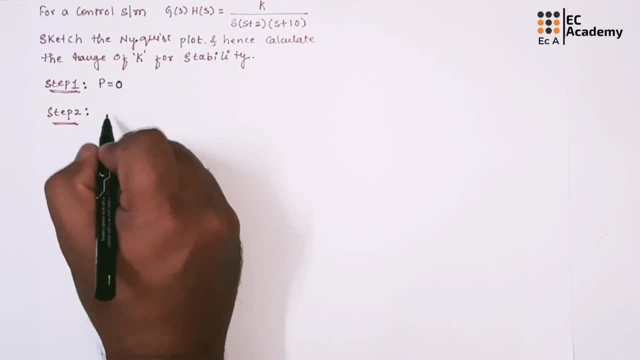 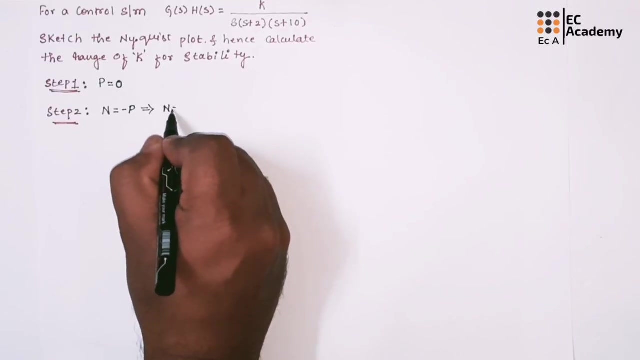 will be 0.. In the second step we need to take, number of encirclements of critical point in F plane will be equal to minus p. Since p is equal to 0, we can say n is equal to 0. Hence we can say: for a system to be stable, the number of encirclement of the 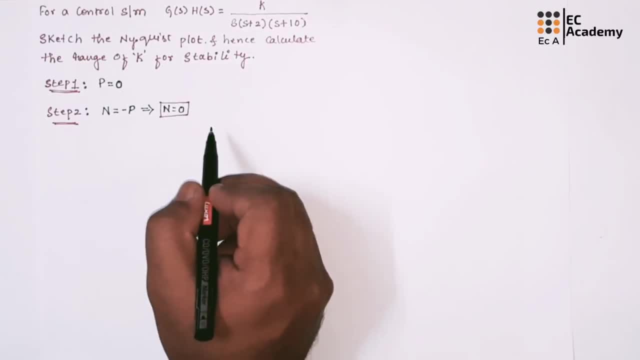 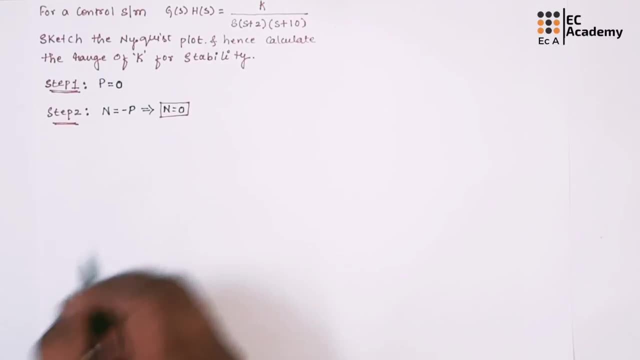 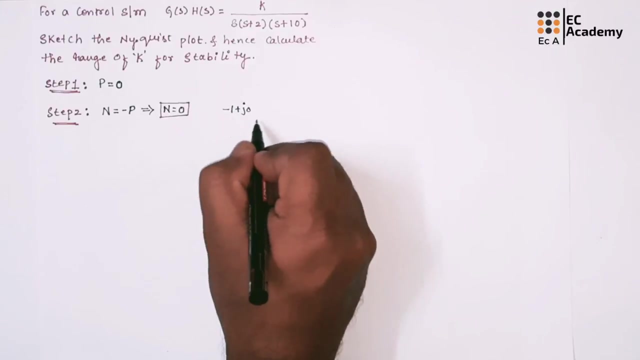 critical point should be 0. So the critical point should not be encircled in F plane for the system to be stable. If we say critical point which is nothing but minus 1 plus j is 0. So this point should not be encircled in the Nyquist plot which we 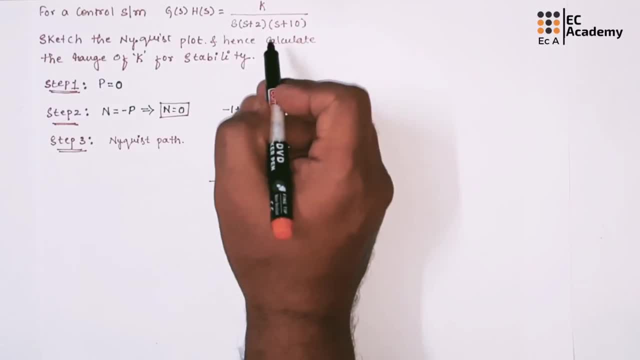 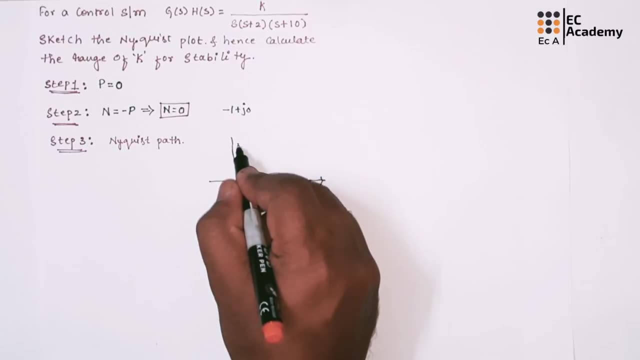 draw. Now, let us draw the Nyquist plot for the given transfer function. Since there is one pole at the origin, so we can write the Nyquist plot like this. So we can draw Nyquist plot here. So at the origin we are having one pole, So this path should not touch that pole. 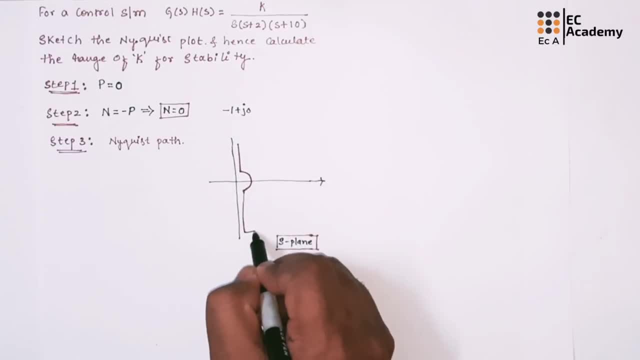 and we need to draw like this. So radius of this semicircle will be: r is equal to infinity, So this point is j 0 and this is minus j 0. So these two points are very close to this origin. So that is why we take that as. 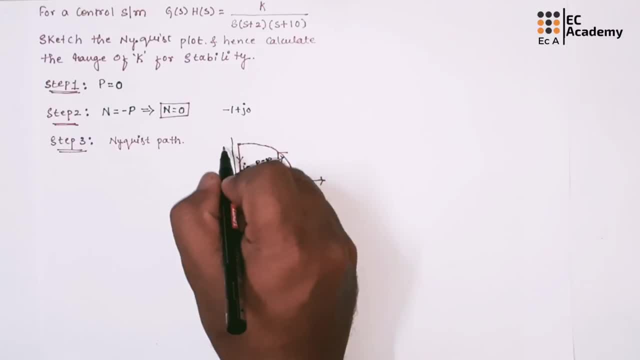 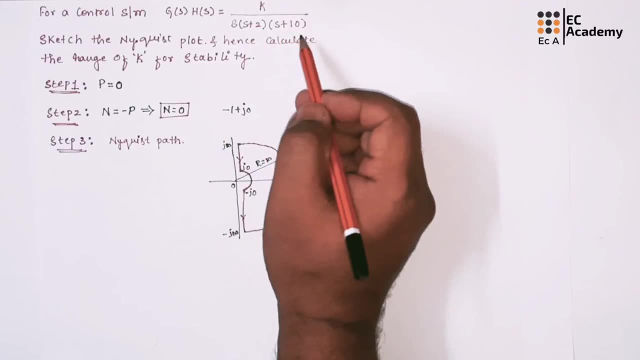 j 0 and minus j 0. So here it will be j infinity and minus j infinity, So in a given transfer, if we do not have any pole at the origin. so this path will write a straight line like this: 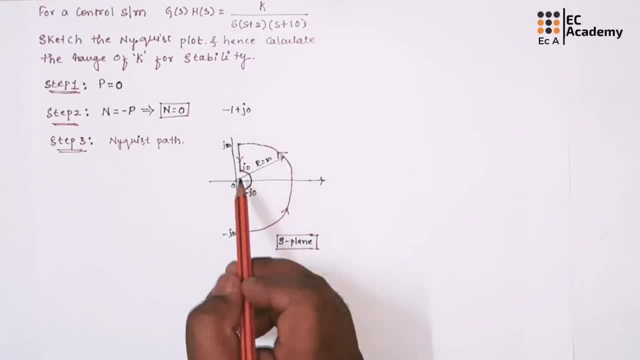 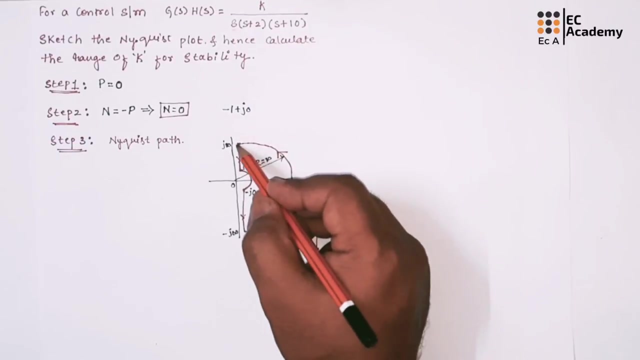 So since we are having one pole at the origin, so here the path should not trace that point at the origin. So that is why we have written a semicircle here. So you need to remember this: If there is no pole at the origin, at that case you can write this path in a straight line without 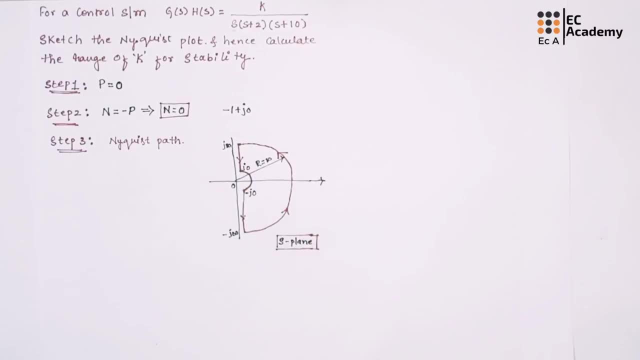 writing this curve like this for other problems. So here we can identify four sections. This is one section, section 1.. Here this is section 2.. This is section 3, this line. So this curve is section 4.. 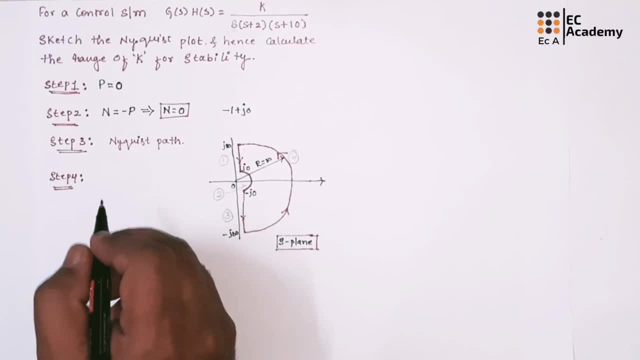 In step 4, we need to find magnitude and phase. For that we need to replace s with j omega, So we can write g of j omega into h of j omega is equal to k divided by j omega into 2 plus j omega, into 10 plus j omega. So from this we can find the. 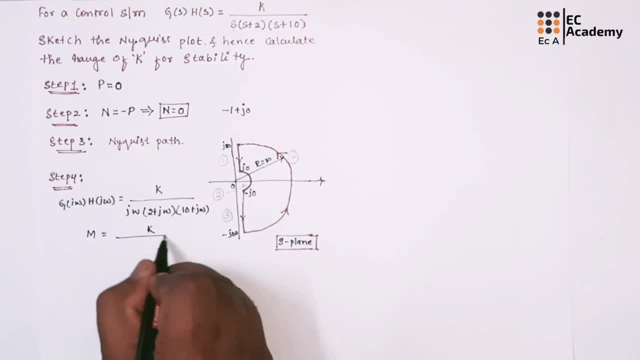 magnitude as k divided by square root of 4 plus omega square. So for this omega value we can write that as square root of omega square, So it will be omega into. so for this term it will be square root of 100 plus omega square And phase value. we can find that as tan inverse of 0 divided. 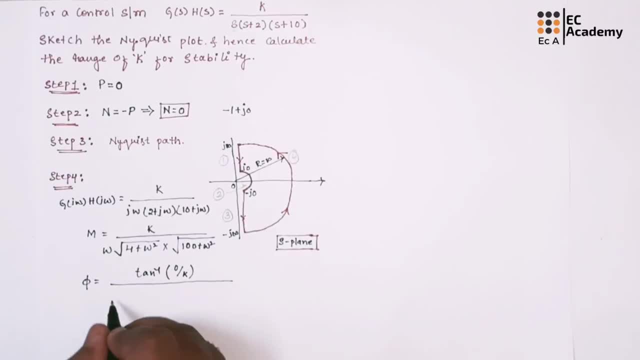 by k whole divided by tan inverse of omega divided by 0,. tan inverse of omega divided by 2, tan inverse of omega divided by 10.. It will be minus 90 degree For the denominator part. it will be minus tan inverse of omega by 2, minus tan inverse of. 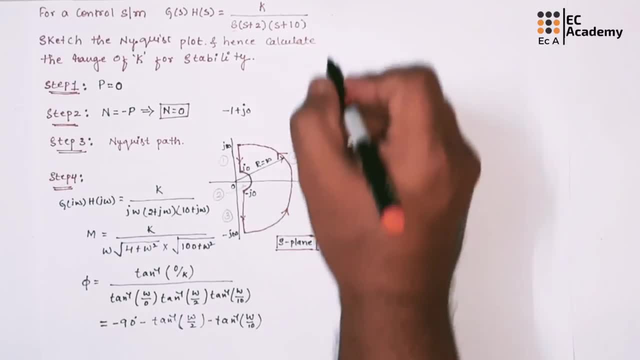 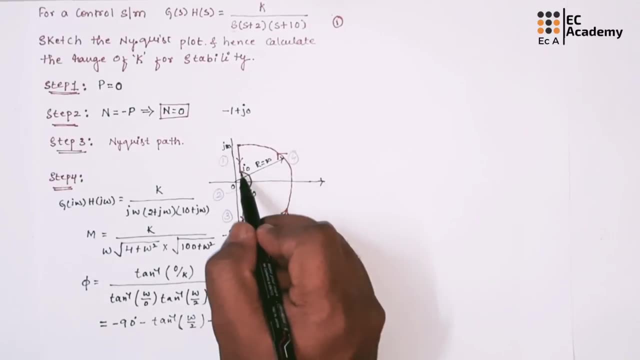 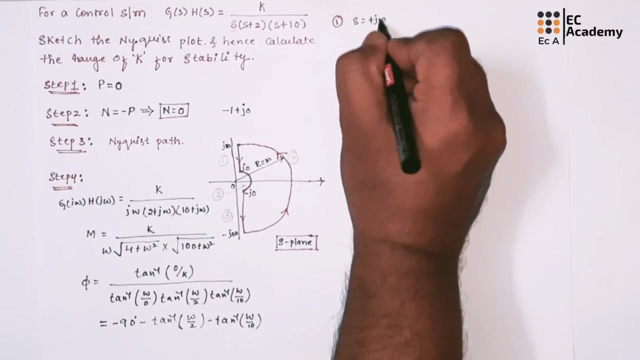 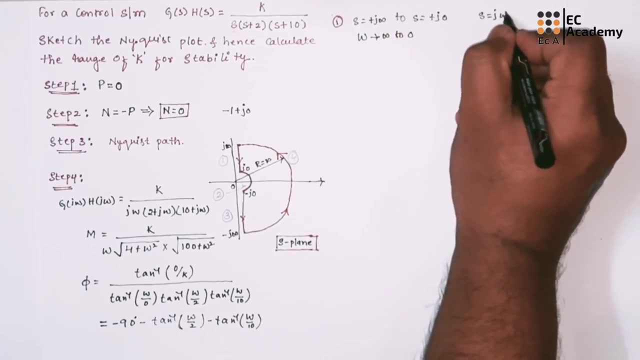 omega by 10.. Now let us consider section 1.. This section 1 starts at j, infinity and it ends 30. So we can write: s is equal to plus j, infinity to s is equal to plus j 0. So omega value will be from infinity to 0,. so here we know, S is equal to j omega. so 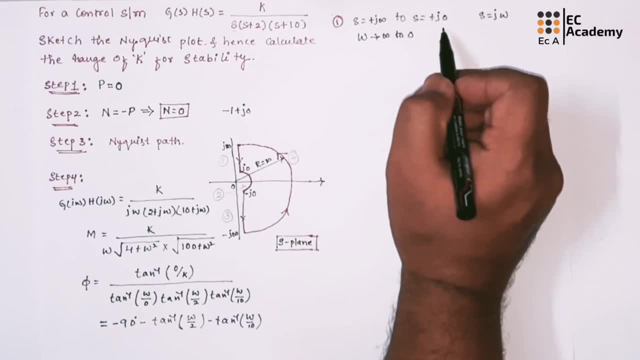 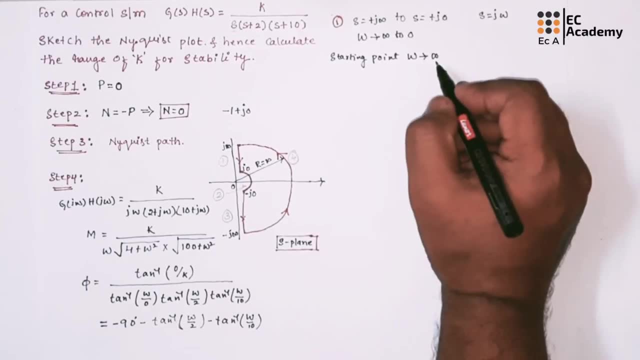 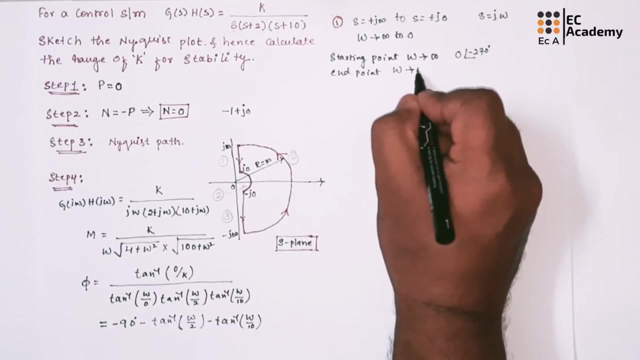 omega value will be from infinity to 0.. So starting point will be at omega is equal to infinity. so if you substitute omega is equal to infinity here, we will get magnitude as 0 and phase as minus 270 degree, and endpoint is at omega is equal to 0. 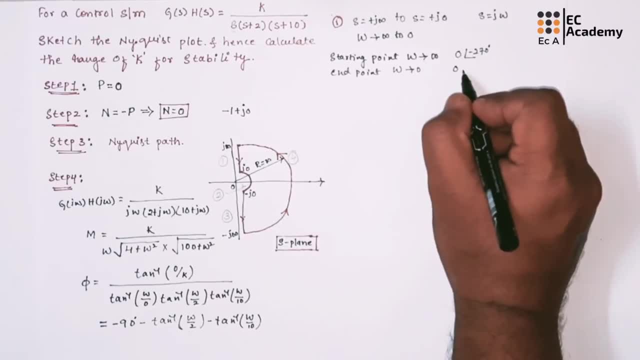 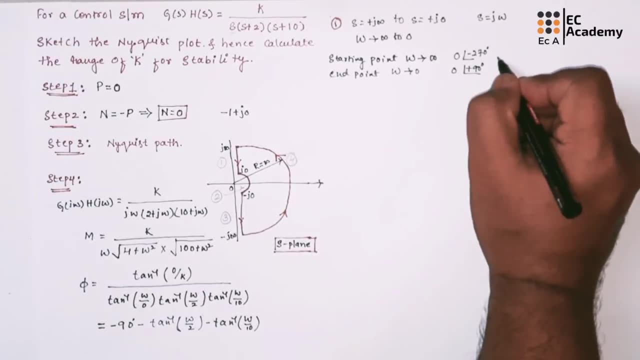 So at that case magnitude will be 0 and phase will be plus 90 degree. So here there will be anti-clockwise rotation of 180 degree. So we will get plus 180 degree, so which means we are having anti-clockwise rotation. 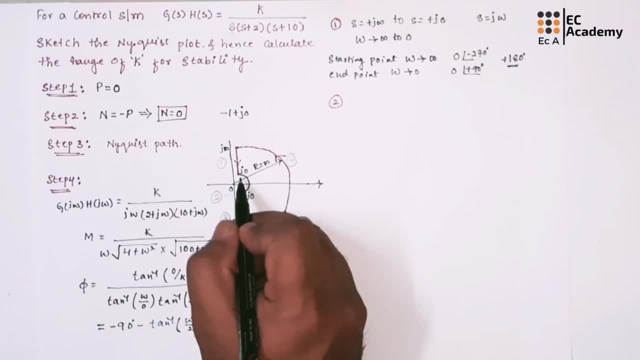 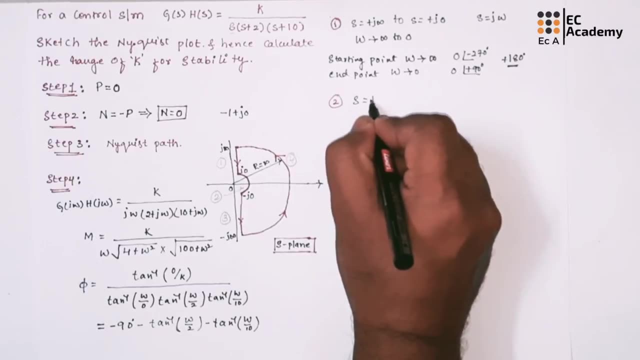 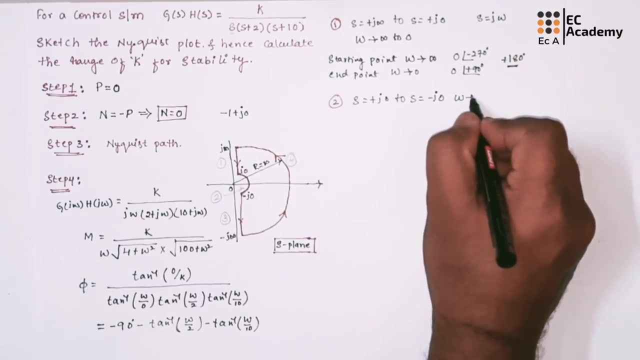 If you consider section 2, it is starting at j0 and it is ending at minus j0.. So S is equal to plus j0 to S is equal to minus j0.. So omega value range from 0 to minus 0.. 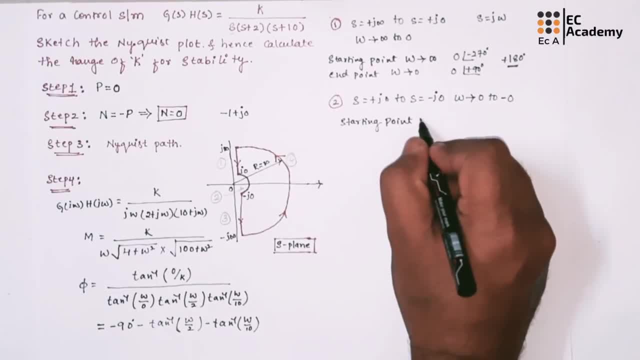 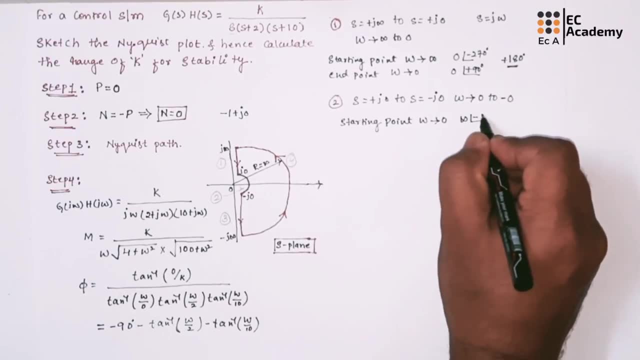 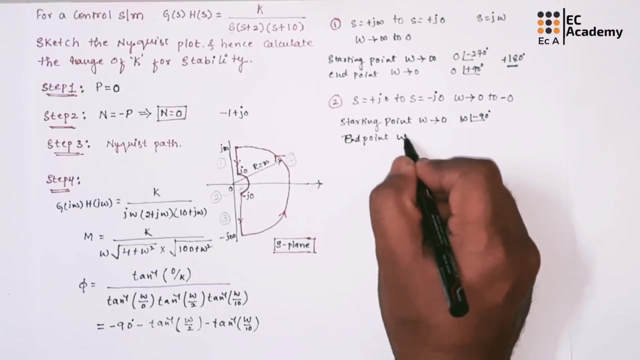 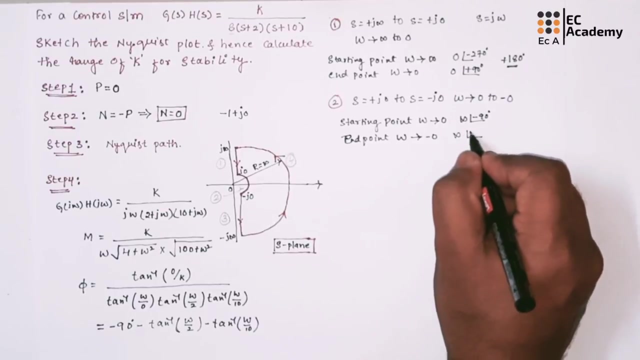 So here starting point will be At omega is equal to 0, for this we will get magnitude as infinity, phase as minus 90 degree, and terminating point or endpoint will be at omega is equal to minus 0, for that magnitude will be infinity and phase will be plus 90 degree. 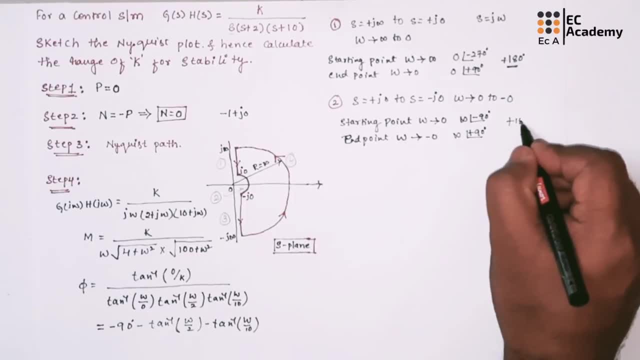 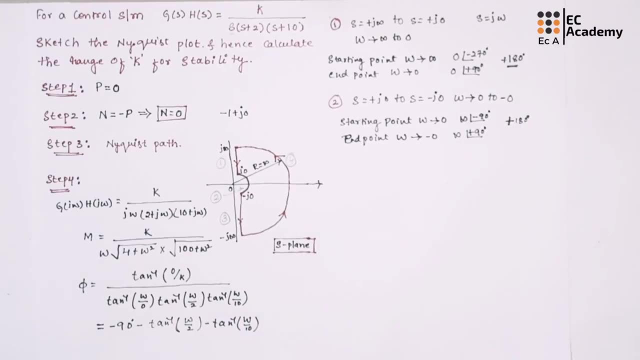 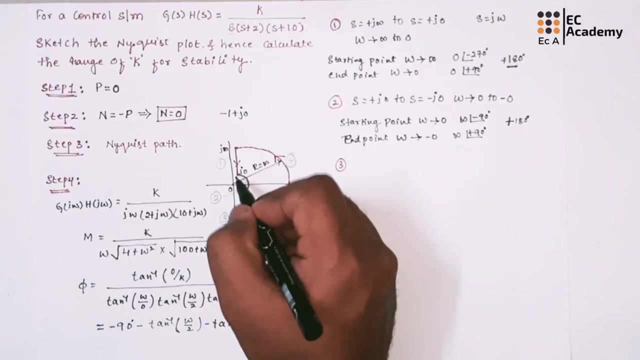 Again, here there will be difference of plus 180 degree. So that's why There will be rotation in anti-clockwise direction for plus 180 degree. Now, if you consider section 3, this section 3 is mirror image of section 1.. 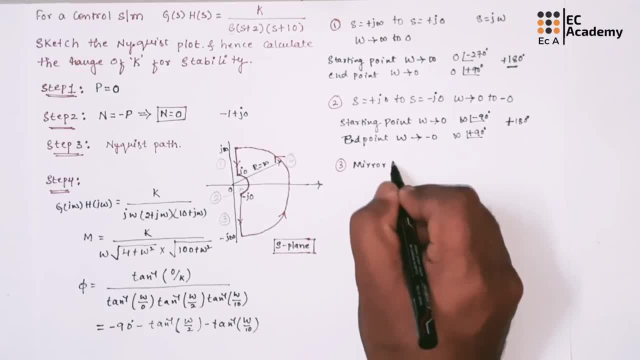 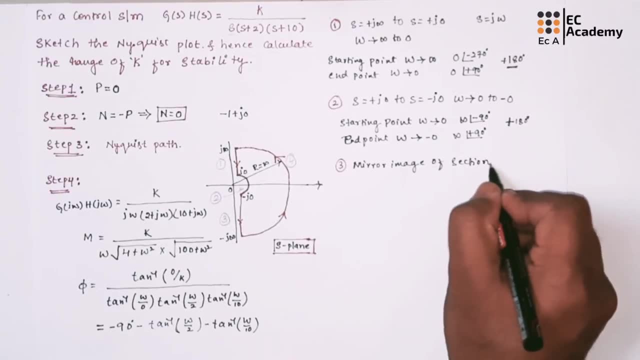 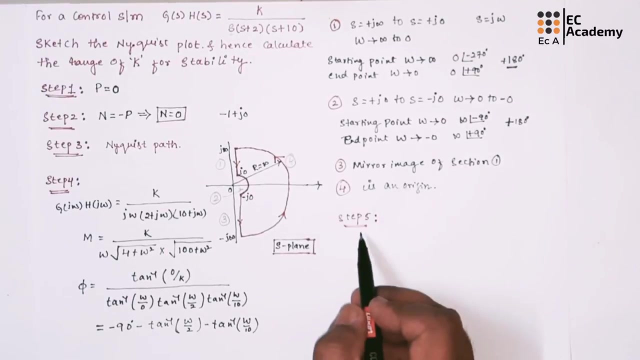 So it is mirror image of section 1.. If you consider section 4.. So section 4. Is an origin In step 5, we need to rationalize this transfer function. To rationalize the transfer function, so we need to multiply and divide with the complex. 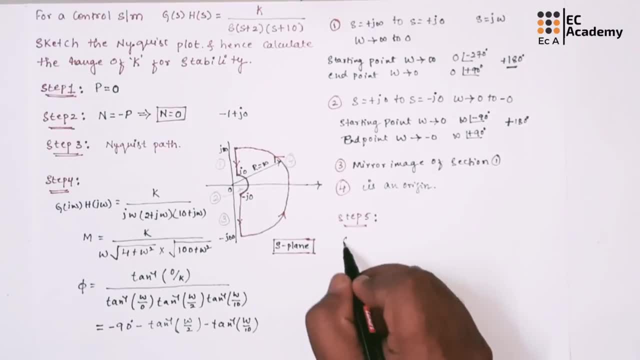 conjugate of denominator term. So we can write g of j omega into h of j omega will be equal to. first let us write the denominator part, So it is j omega into minus j omega into 10 plus j omega into h of j omega into h of j. 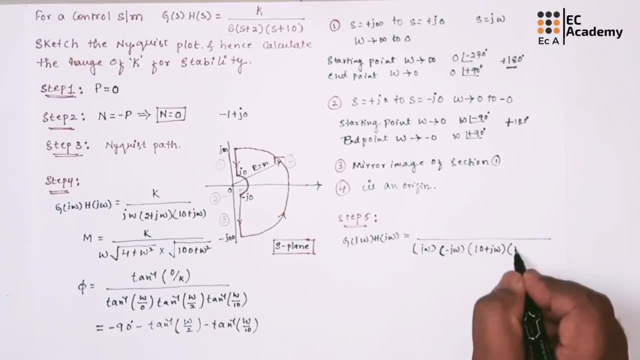 omega. So 10 plus j omega into 10 minus j omega, into 2 plus j omega, into 2 minus j omega. So in the numerator k term we will take and we will write the complex conjugate of denominator which is minus j omega, into 10 minus j omega, into 2 minus j omega. 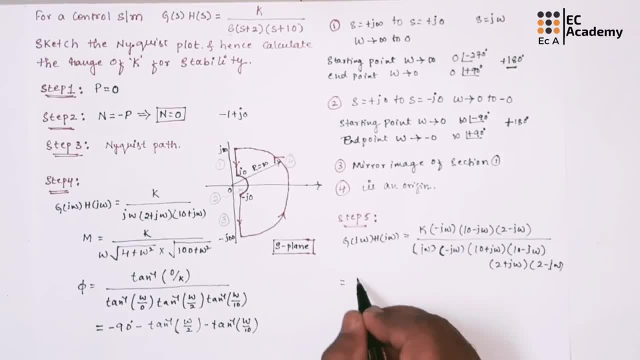 So if you simplify the numerator, we will get minus k j omega into 20, minus 12 j omega minus omega square divided by so if you multiply the denominator part, we will get omega square into 4, plus omega square into 100 plus omega square. Now here let us separate the real term and imaginary term. 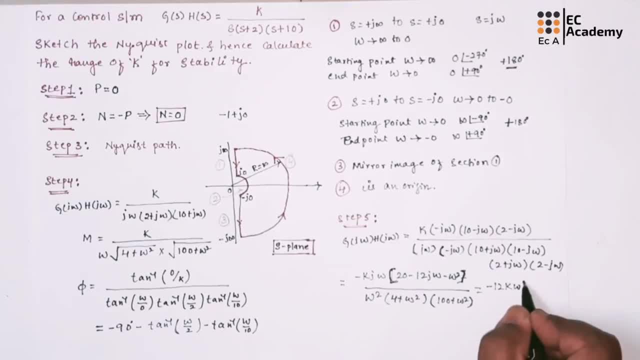 So we can write: minus 12 k omega square, which is the real part in the numerator divided by this denominator term. So d I have written so, which is this denominator term, minus k into j omega, into 20, minus omega square, whole divided by denominator. So this term is the. 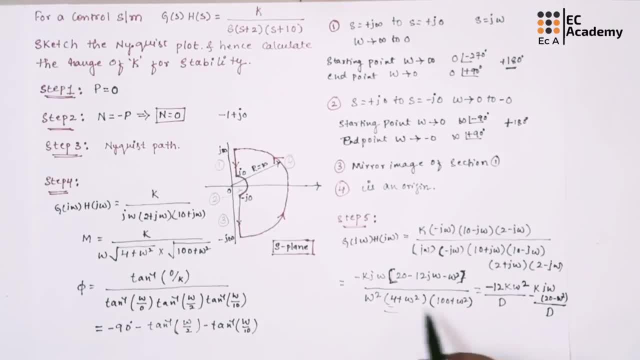 imaginary part of numerator Divided by denominator term, which is represented by d. So here what we need to do: we need to equate the imaginary term to 0.. So we can equate omega into 20. minus omega, square is equal to 0.. 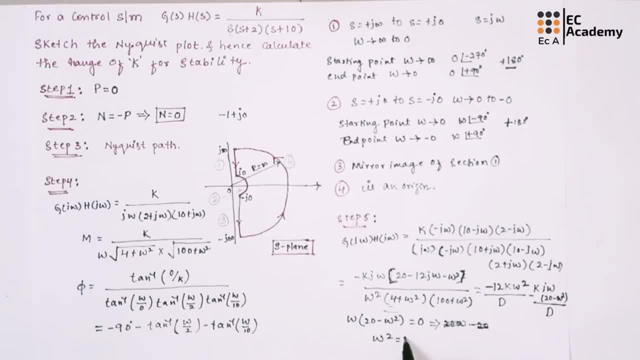 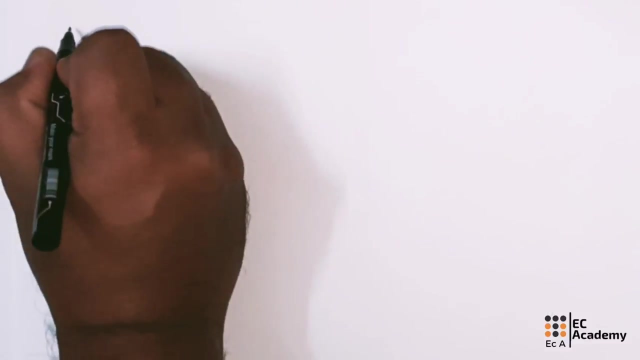 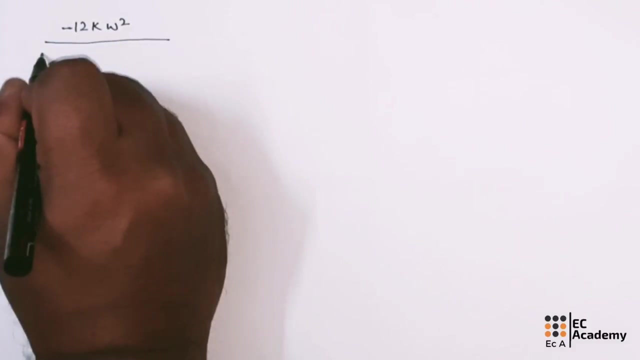 From this we can write: omega square is equal to 20.. So omega is equal to square root of 20.. So this is omega pc And it is phase crossover frequency. We got the real part as minus 12 k omega square whole divided by omega square into 4 plus omega. 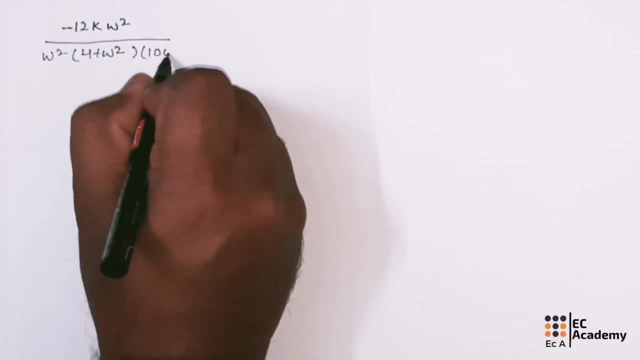 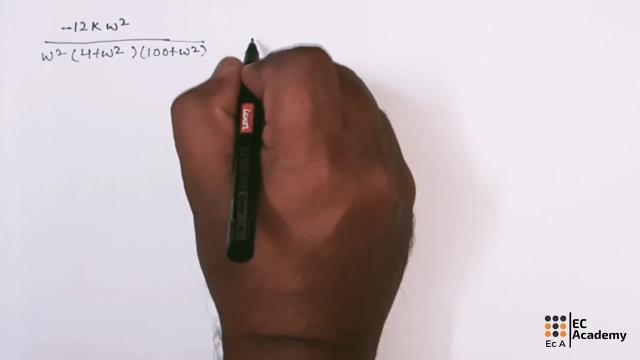 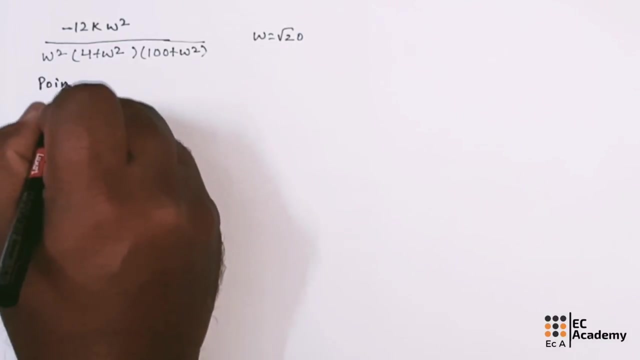 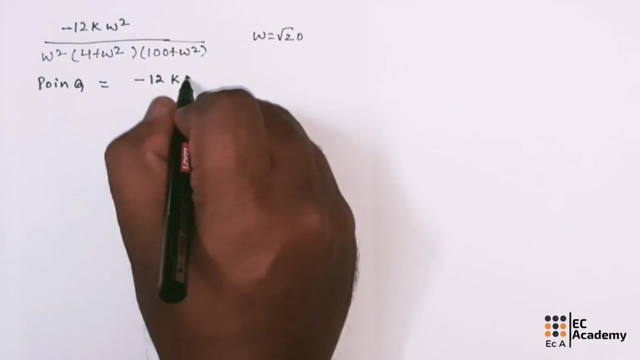 square into 100 plus omega square. So here, if we substitute the value of omega, which is omega is equal to square root of 20.. So we will get point Q on new F plane, So which will be equal to minus 12K into 20 divided by 20, into 20 plus 4. 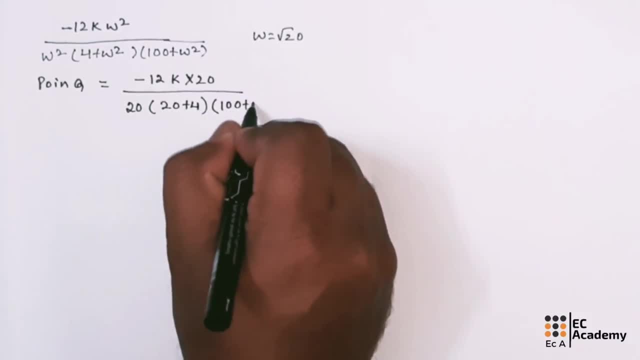 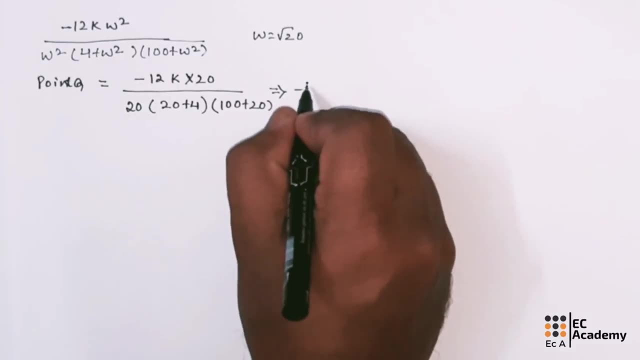 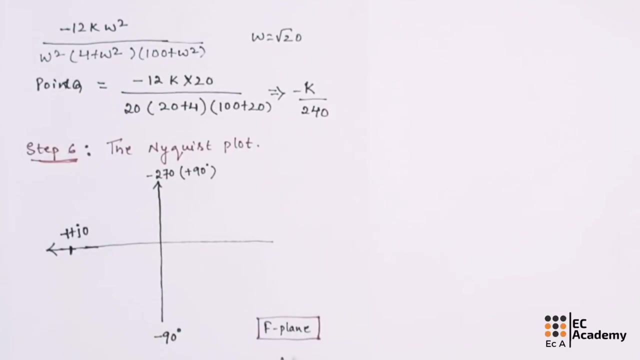 into 100 plus 20.. So we will get the value of point Q as minus K divided by 240.. Now let us draw the Nyquist plot in new F plane. So for this the starting point will be at omega. 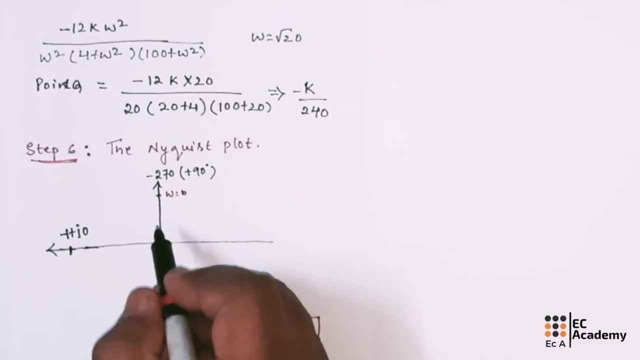 is equal to infinity and terminating point is at omega is equal to 0.. So if we consider section 1, starting point is at omega is equal to infinity, end point is at omega is equal to 0.. So here there will be a rotation of plus 180 degree in anticlockwise. 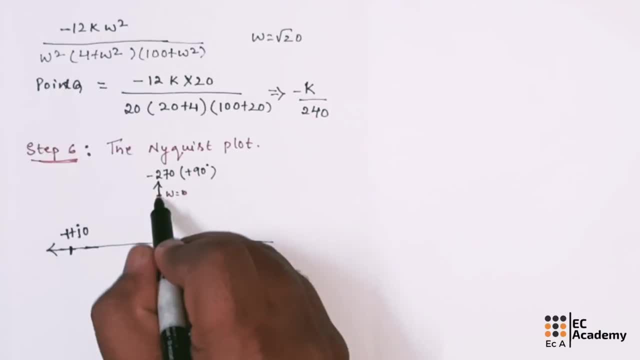 So we can write the plot like this. So this is in anticlockwise direction. Section 3 is the mirror image of section 1.. We will have a path like this: Here it will terminate at omega is equal to minus 0.. So here it will terminate at omega is equal to. 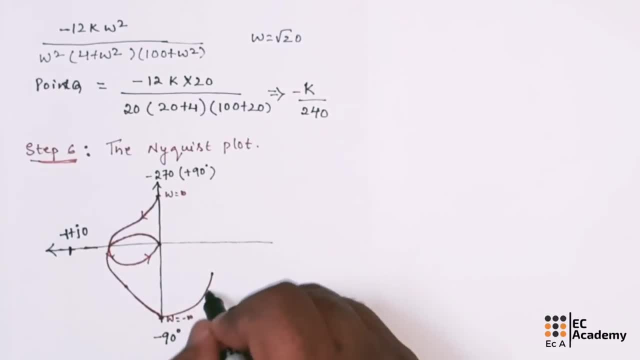 minus 0. So here it will terminate at omega is equal to minus 0. So here it will terminate at omega is equal to minus infinity. So we can draw the section 4 as it is. So this is the critical point, And since n is equal to 0, the critical point will not be. 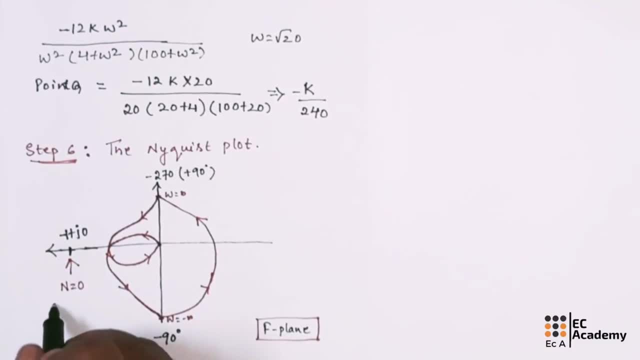 encircled, So that is why the system will be stable. So here we can write 0.0 and here this is 0.0.. So here we can write 0.0 and here this is 0.0.. So here we can write 0.0.. 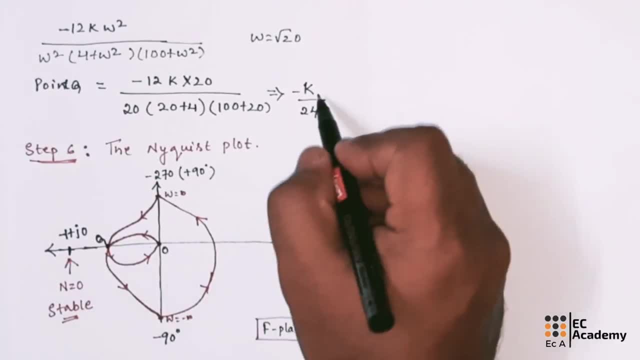 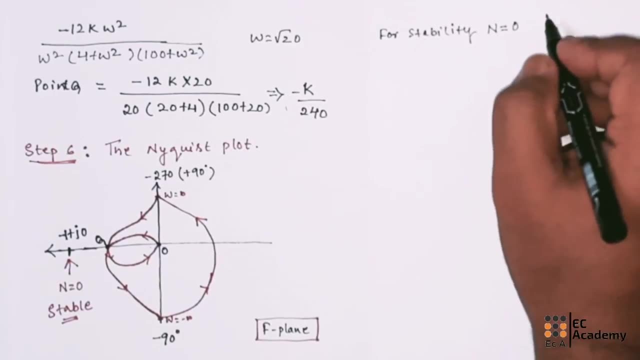 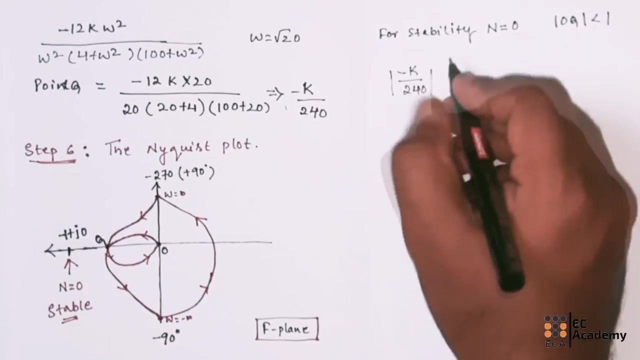 This is point Q. So this is the value which we have found here For stability. n will be equal to 0 and magnitude of Q and 0 should be less than 1.. So we got this value as minus k divided by 240.. It should be less than 1.. Therefore, 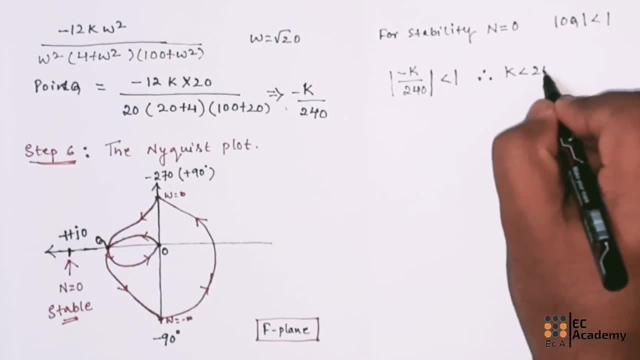 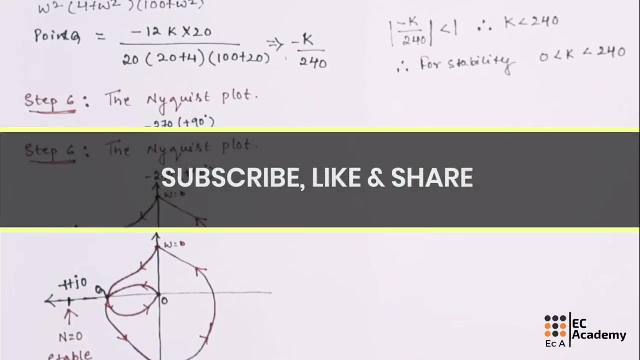 from this we can write: K should be less than 240.. Therefore, for stability, K should range between 0 and 240.. This is about the problem on Equest plot. Hope you have understood the topic. Thank you.